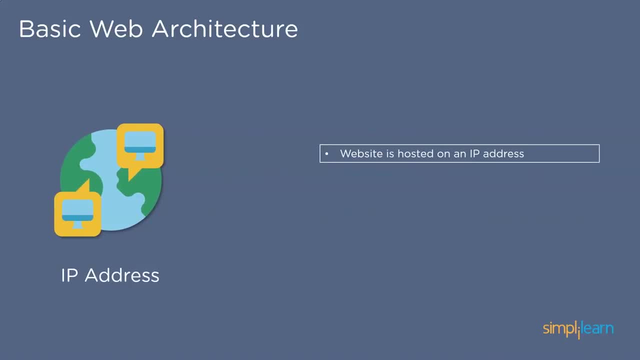 Now a website is hosted on an IP address, We put a domain name over that IP address, the same way we put names over people's phone numbers. When you type a domain name in the browser, it will give you the server call. The server will then send over the website. 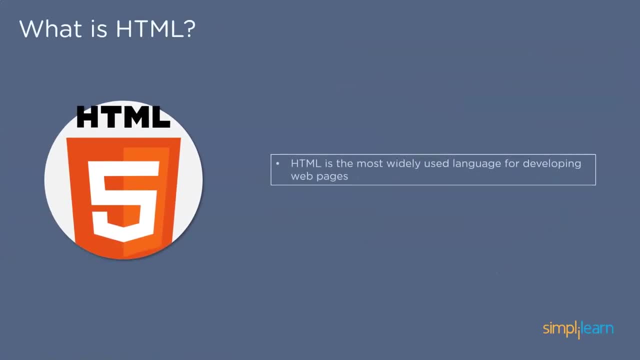 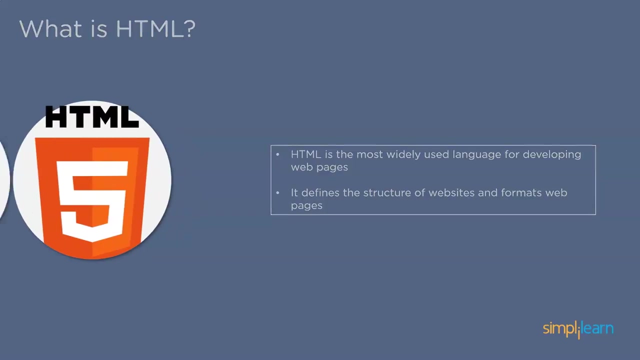 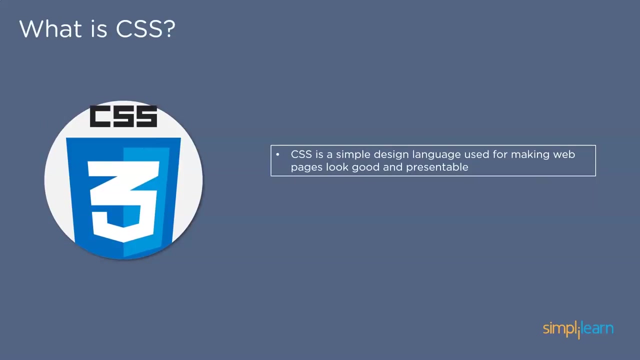 to you Next, what is HTML? HTML is the most widely used markup language for developing and structuring web pages on the internet. It defines the structure of websites and formats these web pages. So what exactly is CSS, then? Now, CSS is a simple design language used for making web. 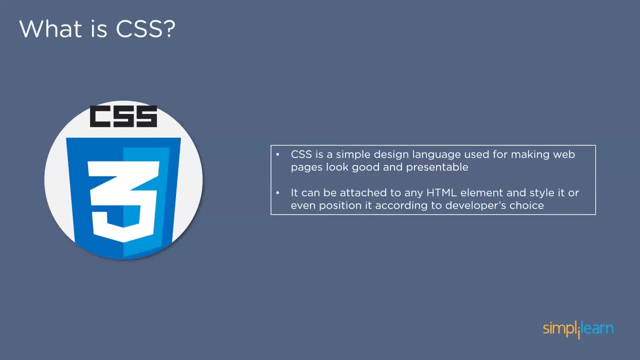 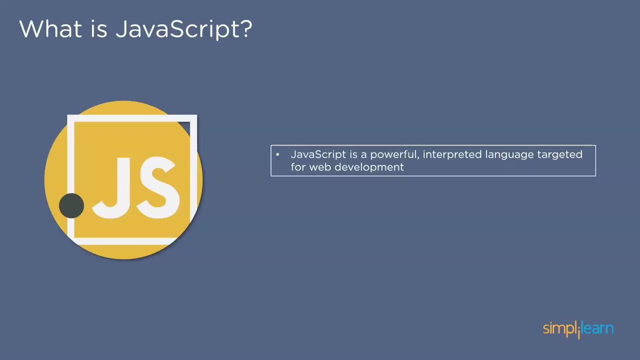 pages look more beautiful and presentable. It can be attached to any HTML element to style it or even position it according to the developer's choice. Then you must be wondering: what exactly is JavaScript Now? JavaScript is a powerful interpreted language targeted for web development. It is used for making web pages interactive. 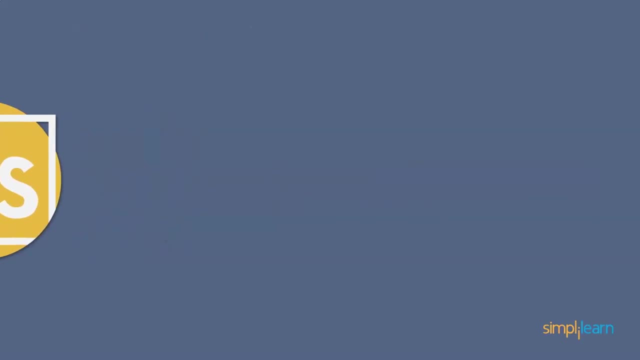 and bringing the web pages to life. So now let's create your first website Now. HTML, short for hypertext markup language, is the coding standard for documents designed for web browsers consisting of a series of elements or tags and which can be used to. 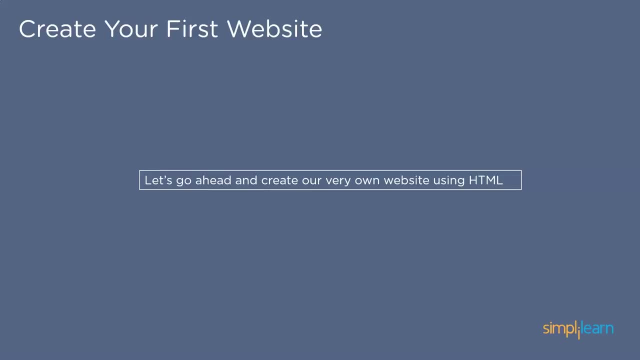 structure a web page Right. So these elements can include headings, paragraphs, documents, div containers, tables and more. HTML tags are nested, meaning there are opening and closing tags with the content in between those tags. So now let's write a simple HTML code that will help you understand the basics of the 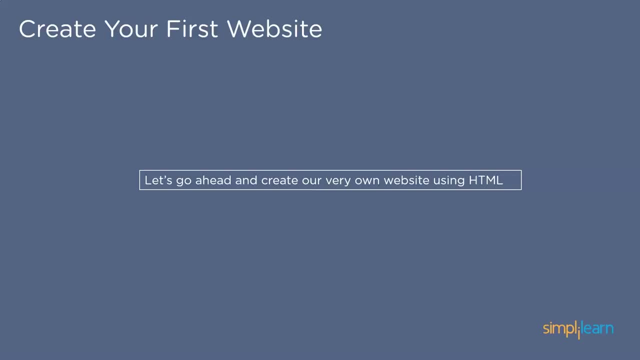 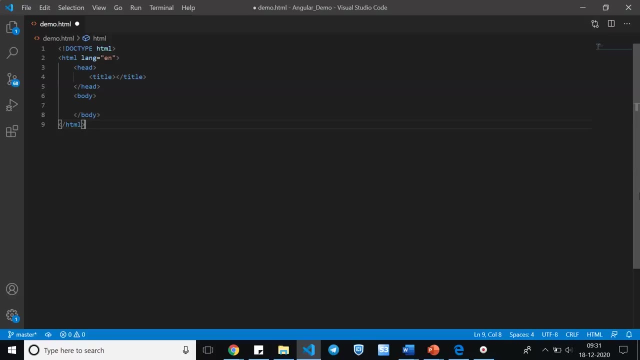 language. So for this I'm using the text editor, that is, Visual Studio Code. You can go ahead and download this text editor from their official website. So here I've created a simple dot HTML file in my VS code and I've added the initial HTML files. 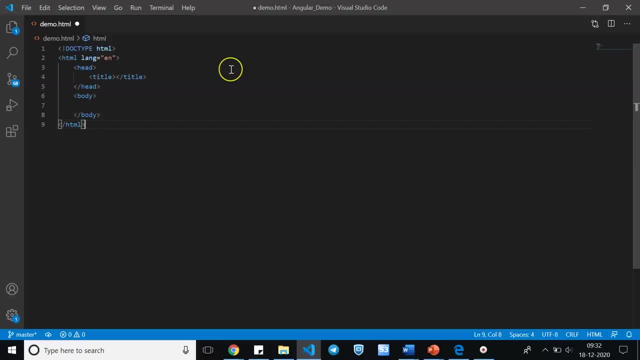 Now let me explain to you one by one. Now, doc type is not so much of a tag, but it is more of an instruction. Now this indicates the browser that the document type to be served to the user is in fact an HTML document. Now, this doc type instruction should always be. 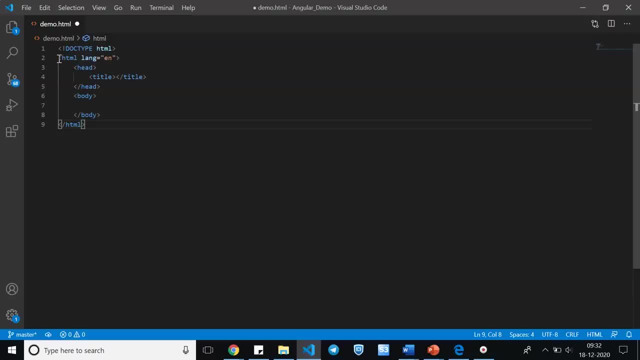 included at the very top of your HTML page. Next up, you have the HTML tag that is used to contain all the web pages' HTML code, right? So it contains an opening and closing tag with the contents in between them. The HTML tag can also have attributes. Now for. 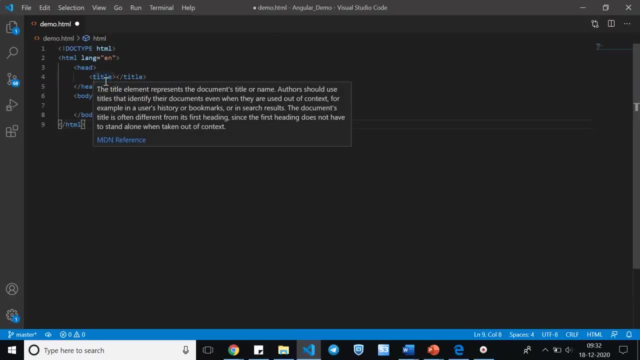 example, there's the lang attribute allowing you to specify the spoken language of the contents of the page. Followed by the HTML tag, there's the head tag. Now, this is the first section of the code that contains all of the information about the web pages' properties. 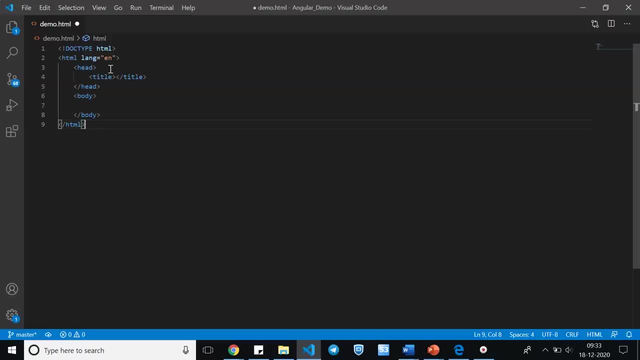 links and more. It could have pages, title description, additional meta tags and CSS code. So here I've used the title tag And let's give a title, say HTML in 10 minutes. Alright, You can also add CSS to the head tag. 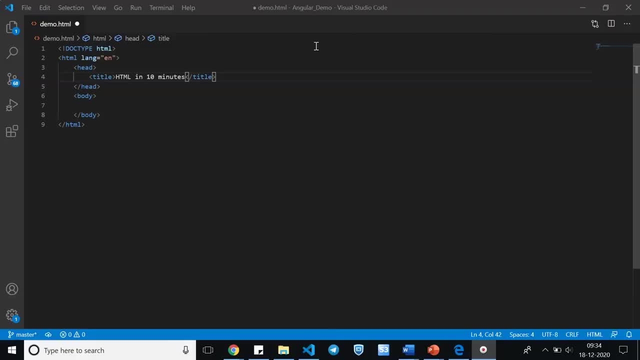 by using the style tag and change the display styles of HTML elements that are being used. The next section is the body tag. Now the body tag contains all the displayable contents of your web page, including headings, paragraphs, div containers, tables and more. Now the HTML. header tags are used to display all the contents of your web page, including headings, paragraphs, div containers, tables and more. Now, the HTML header tags are used to display all of the contents of your web page, including headings, paragraphs, div containers, tables and more. 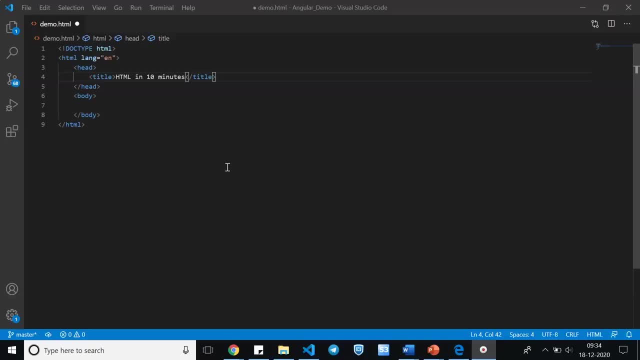 There are several types of headings available for developers to add to a web page. Alright, So first up, let's have a look at them. I'm going to create a simple H1 heading tag And the message I'm displaying is: this is the first heading. 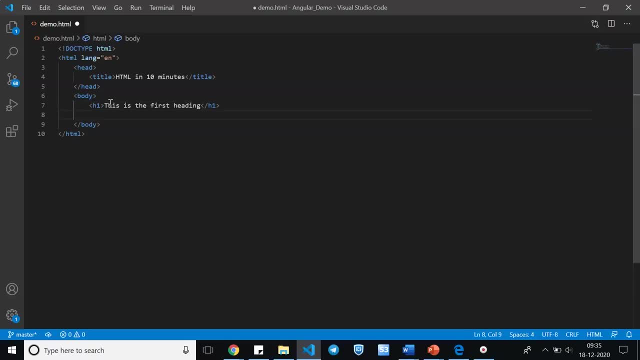 Alright, After this, I'm going to add a paragraph tag which creates padding in the top and bottom of the element. So the first heading I'm going to add is a paragraph tag which creates padding in the top and bottom of the element. 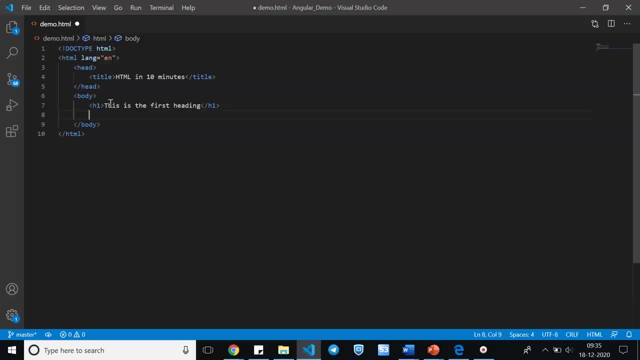 to help separate the text between each paragraph, right? so i'm gonna add a p tag and say this is the paragraph tag. after this, let me add a simple h2 tag, which is another heading tag, and say: this is the second heading, this is the third heading, and you can also add line breaks, which are helpful from time to time. 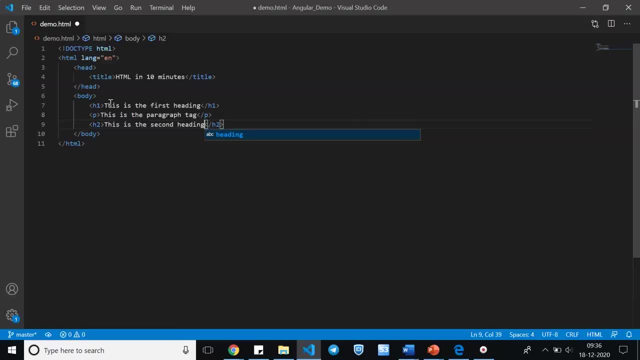 if you want to provide a single line break in your content, you can do so by adding the br tag, so here let me just add one for better understanding now. the html div tag defines a division or a section in an html document that is used as a container for other html elements. 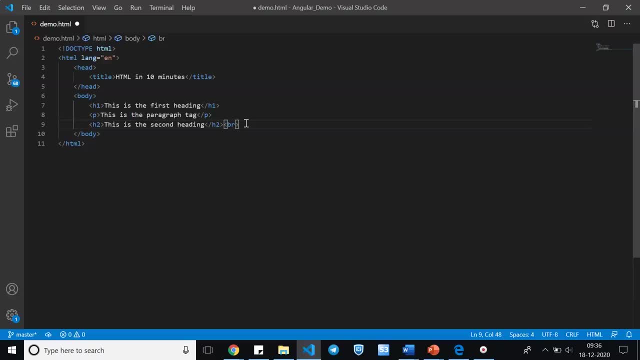 now these elements can include content sidebars, page bars, page headers, footers, etc. This tag is used to apply styles to HTML elements that cannot be added otherwise. We can also make use of the HTML image tag to add images to a web page. Now these images in a web page are: 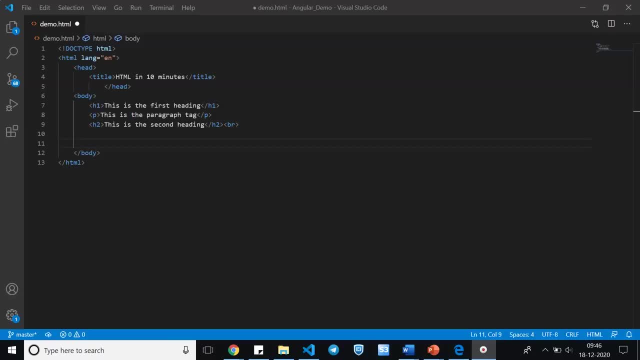 a very common site, and they can make the website look more attractive. So for that we can use the image tag, So let's say img, within which I mention the source. I'm adding the HTML logo, so let me just mention that here, and then I'm going to. 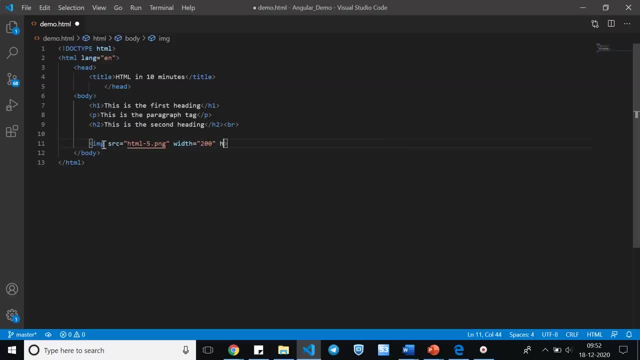 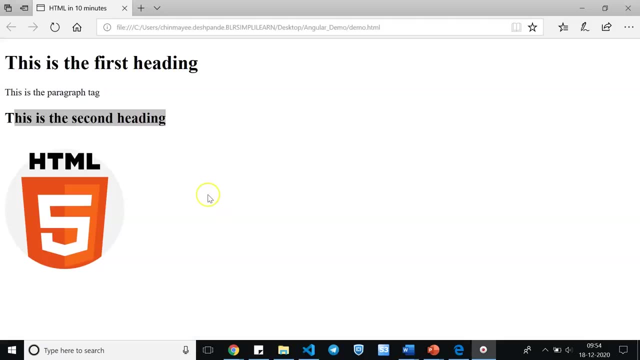 provide width for it and then a specific height. Alright, so when you save the file and when you look at the browser, you can see that the first heading is displayed, then your paragraph tag is displayed, followed by the second heading and then the image. Now let me show you. 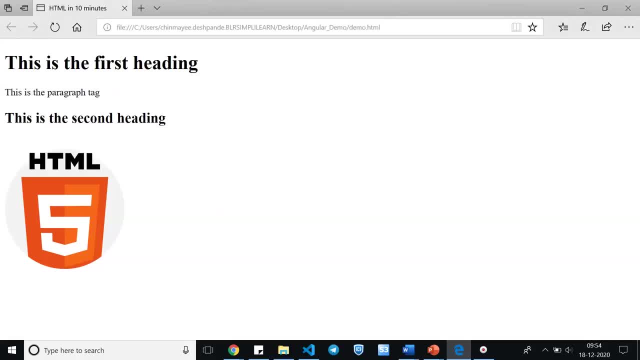 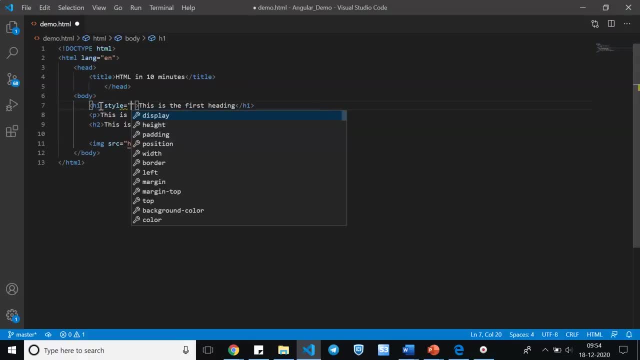 how you can add styles for some of these headings and paragraph tags. So here in back, in my first heading tag, let me just say styles and let me change the font of the content that is being displayed. I'm going to change it to career, new and. 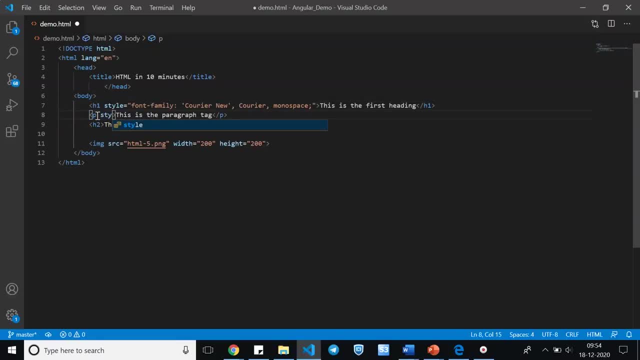 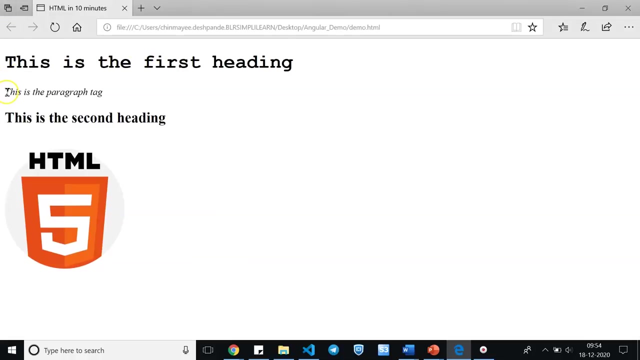 for my paragraph tag. let me display the content in italics. So I'll say font style and make it italics, So let me save this. and when I look at the browser, you can see that the font has changed and so has the font style here. So now we've covered. 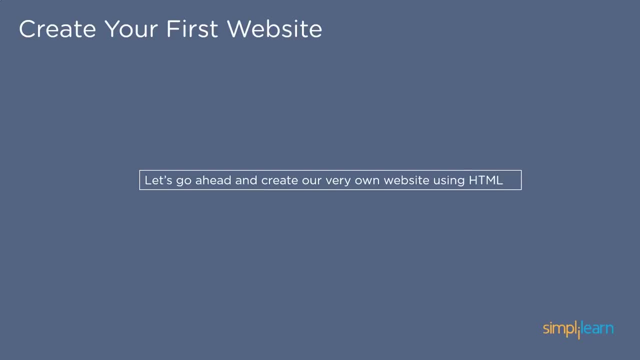 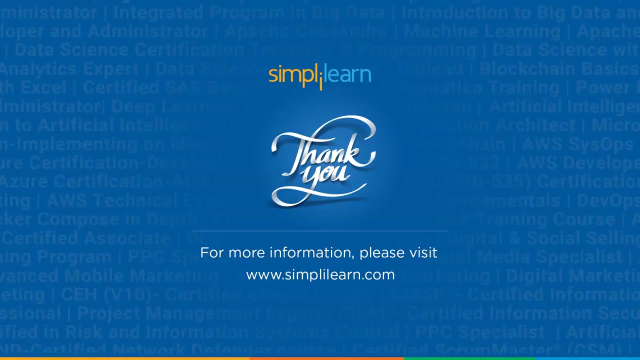 a few important HTML tags used to develop a web page. Now there are many other tags available for almost everything you'd want to add to a web page. So all of these are available on the internet for you and you can use them in your website. So with that we've reached the end of this video. I hope you liked.